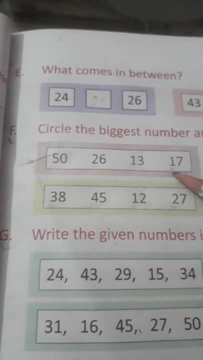 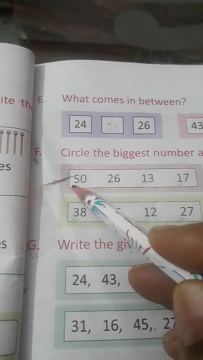 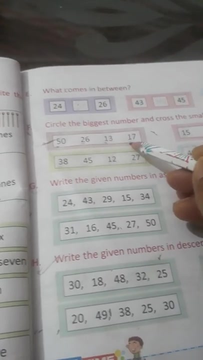 We have to compare the digits at 10th place first. Ok, So in 50 it is 5. at 10th place, in 26 it is 2, in 13 it is 1,, in 17 it is 1.. 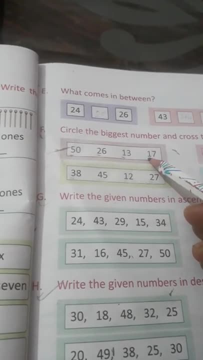 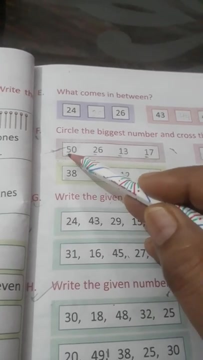 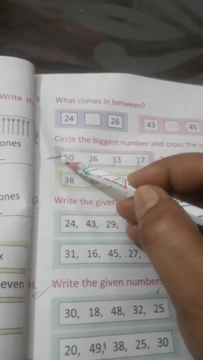 Ok, Which is the greatest number here? 5 is greater than all the 4 numbers. The 5 is the biggest among all the 4 numbers, So it means 50 is the greatest number here. So circle it Like this: 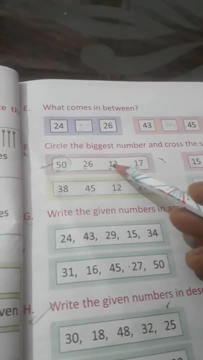 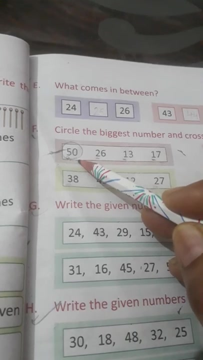 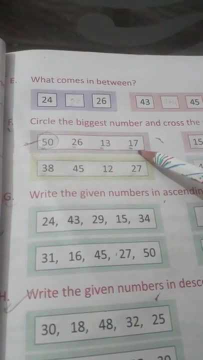 In counting, 50 will come at the end When you see 26,, 13 and 17,. the last number in counting is 50. So 50 is the greatest number. Now we have to find out the smallest number: 26,, 13 and 17.. 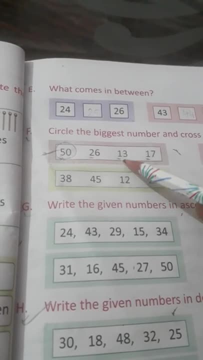 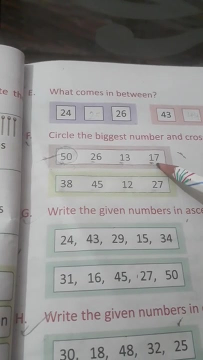 In this also, we will see at 10th place 2, 1, 1.. So, students, if the digits are 10th place, then we have to find out the smallest number. If the digits at 10th place are same in numbers, then we compare the digits at 1st place. 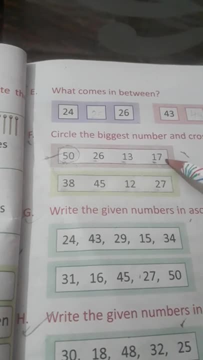 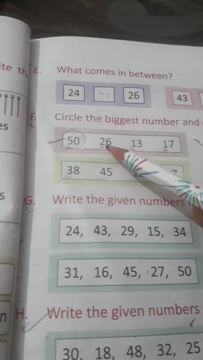 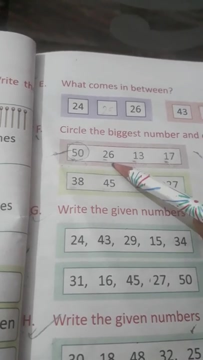 Then we compare the digits at 1st place, Ok, To find out which number is greatest and which number is smallest: 2, 1 and 1.. So 2 is bigger than 1.. Ok, It means 26 can't be the smallest number. 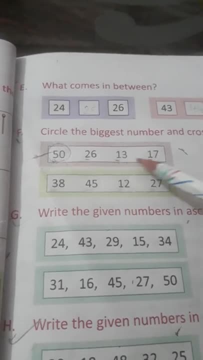 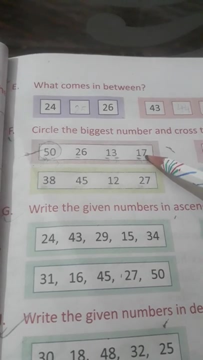 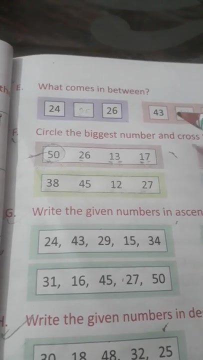 Ok, Now we have 13 and 17. In 13,, 3 is at 1st place and in 17 it is 7. So which is smaller? 3 is smaller than 7.. So it means 13 is the smallest number here. 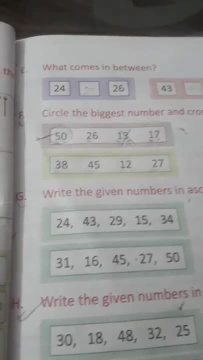 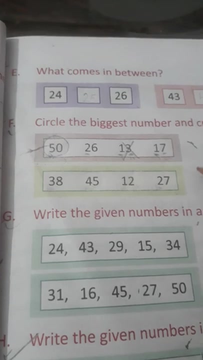 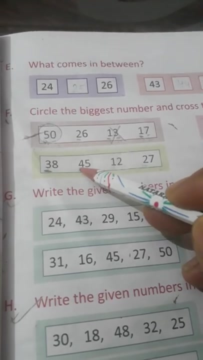 So cross it like this Now: next 38,, 45,, 12 and 27.. Here first see the first number. So we have 3 digits in all the numbers, Here we have 3.. In 45, it is 4.. 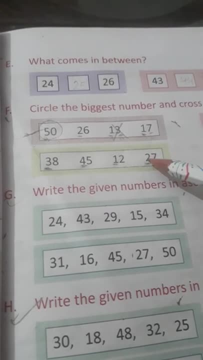 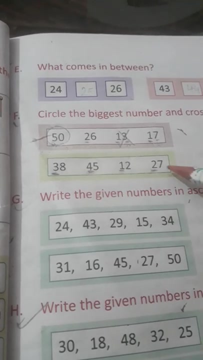 In 12, it is 1.. In 27, it is 2.. So which is the greatest number here? 4 is greater than 3.. 4 is greater than 1.. 4 is greater than 2.. It means 4 is the greatest number here. 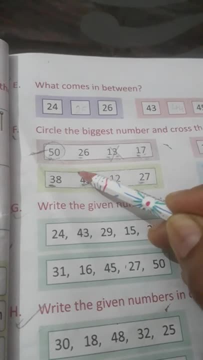 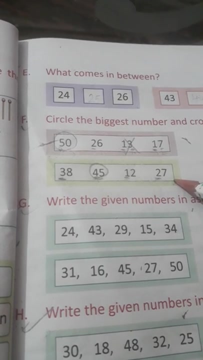 So it means 45 is the greatest number here. So circle it like this: Now we have 38,, 12 and 27.. So we have 38,, 12 and 27.. So when 27 left, we have to find out the smallest number. 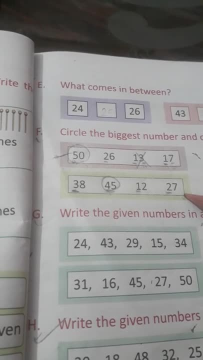 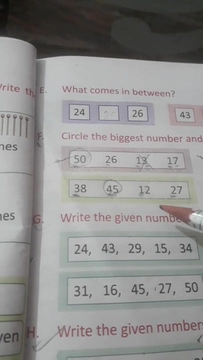 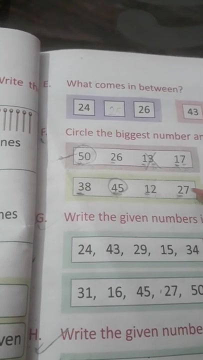 Students. when we recite counting, which number comes first, That number is the smallest number. When we recite counting, the number which comes first is the smallest number. When we say counting 12 comes before 27 and 38.. 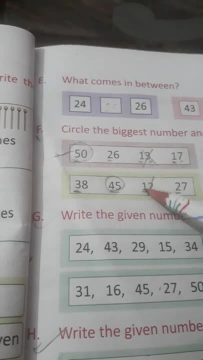 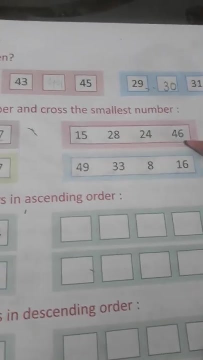 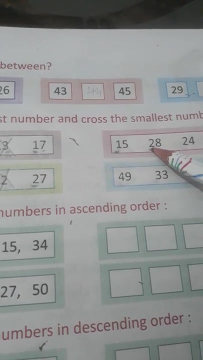 So it means 12 is the smallest number here, So cross it like this. Now: next 15,, 28,, 24 and 46.. Okay, First digit: 1. In 28, it is 2.. In 24, it is 2.. 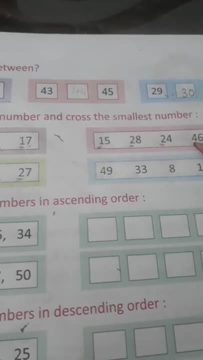 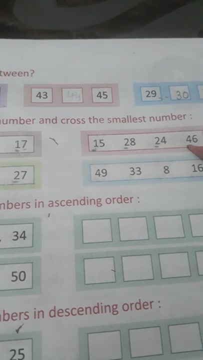 In 46, it is 4.. Okay, Which is the greatest number here? 1,, 2,, 2, 4.. 4 is greater than 2.. 4 is greater than 1.. 4 is greater than 2.. 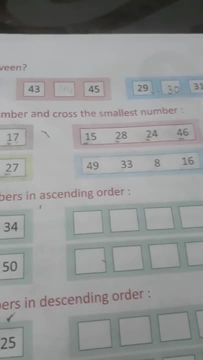 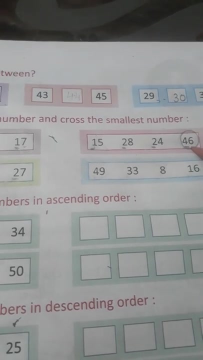 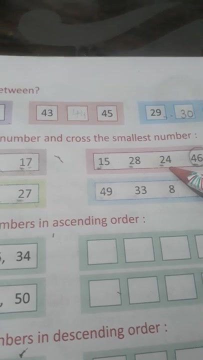 4 is greater than 1.. It means 46 is the greatest number here. 46 is the biggest number here. So circle it like this. Okay, Now we have to find out the smallest number: 15,, 28 and 24.. 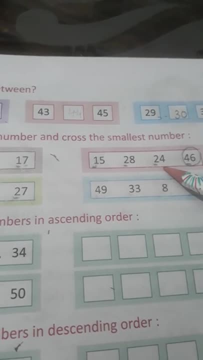 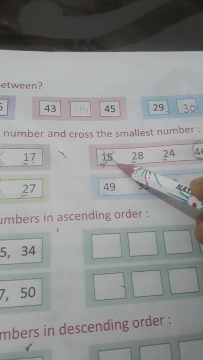 So while counting which number will come first, That is 15.. So cross it It means it is the smallest number here. This is the biggest number here: 4, 3, 3, 4,, 4 and 4, which is 16.. 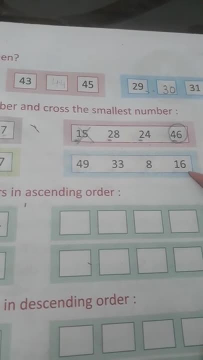 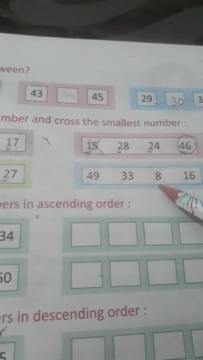 Next 49,8, and 16.. Next 49,8, and 16.. Next 49,8, and 16.. Students, here we have number 8.. Students, here we have number 8.. A single digit number. 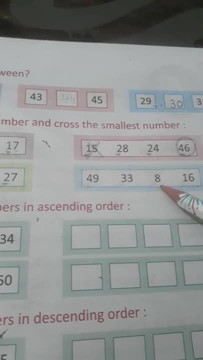 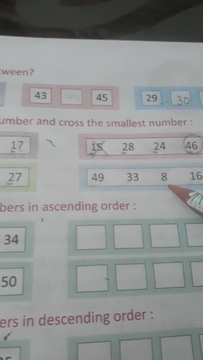 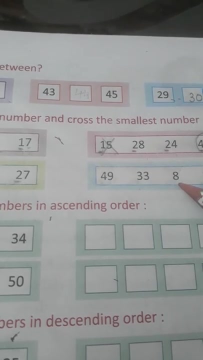 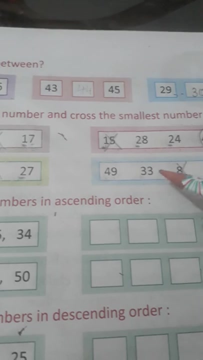 is always smaller than a two digit number. A single digit number is always smaller than a two digit number, which means the two digit number is smaller. So it means 8 is the smallest number here, so cross it. Now we have three numbers left: 49, 33 and 16, which is the greatest number here.